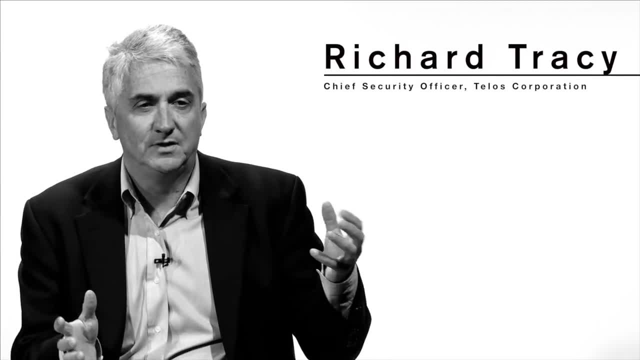 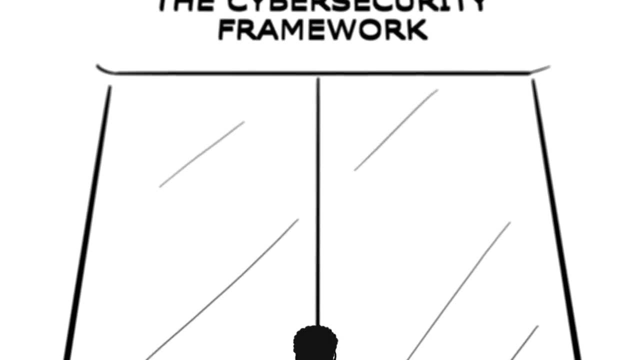 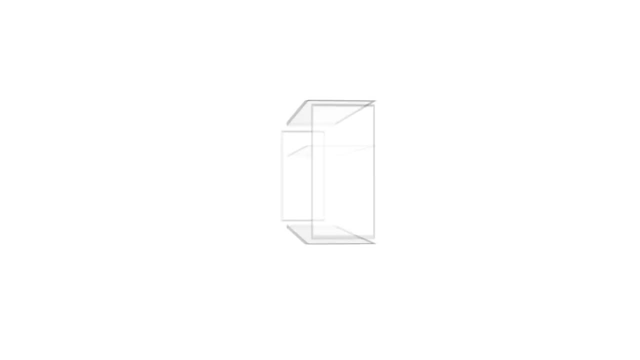 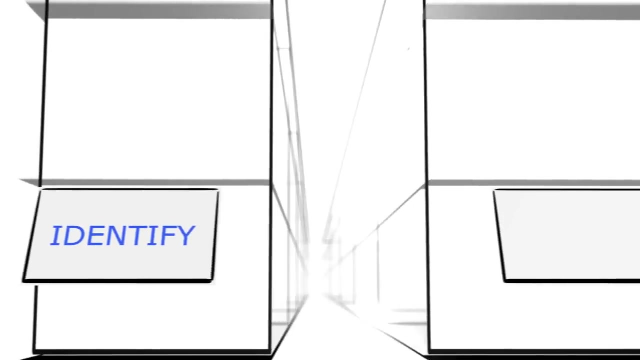 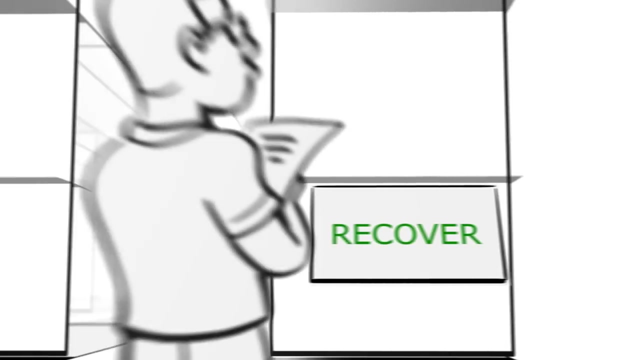 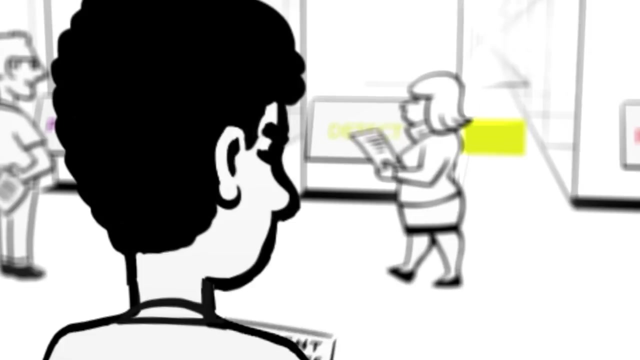 It helps us communicate risk in ways that everyone understands, from the server room to the board room. миллиohn- I think it was at Mn пош, hvor I use two words that I don't use. every word people use in relationships. I wouldn't understand if ones was lips to my eyes. What is it Size is asking folks how long the range of things you can slingshot into your crowd If you can timing that number on a market. what could you do to find the rightっちゃ? What are the areas that we found ourselves both challenged in? assets, organizations that peaked in the way of Быckiva and that area? The strong libel Gaddebag perfect industry, which I believe that that it's the same industry that when there was something that was eatin' about it. that's where it's moving now. So that's things are now movin' along. 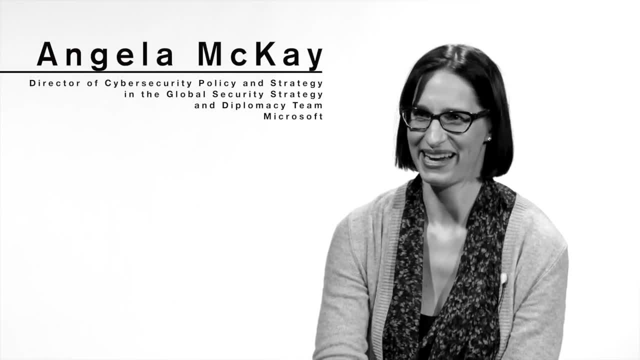 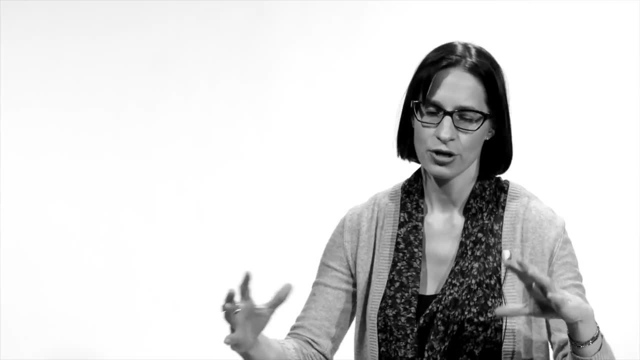 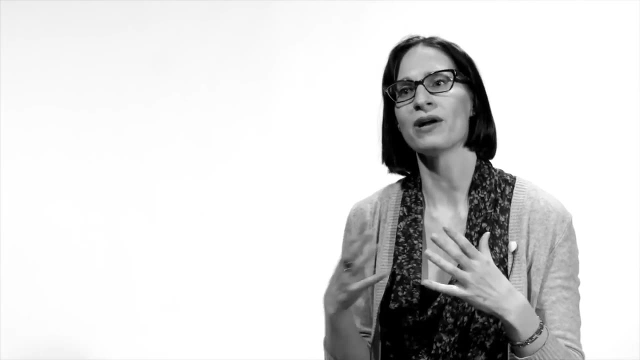 At this pointımız challenged and stimulated by, was building out the detect function. this aligns well with kind of what's been going on in the industry writ large, which is an evolution from kind of a protection kind of mindset to one where there's a recognition that organizations are going to have successful cyber. 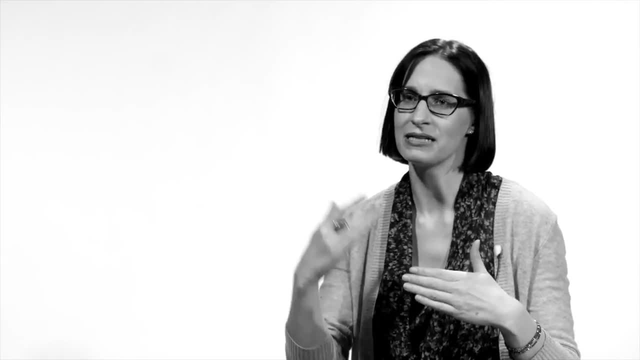 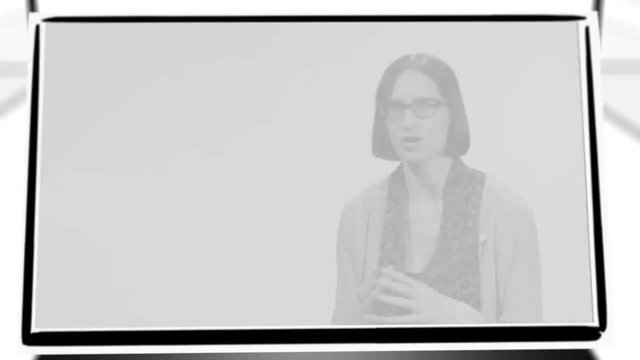 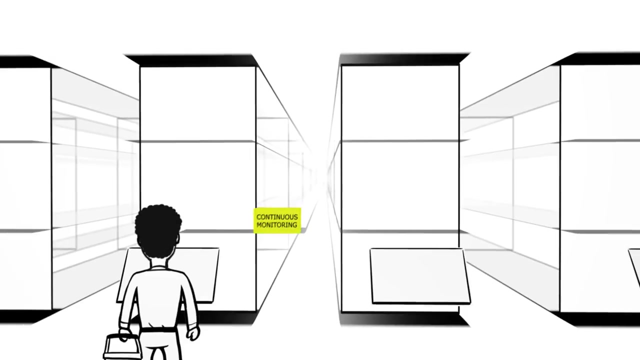 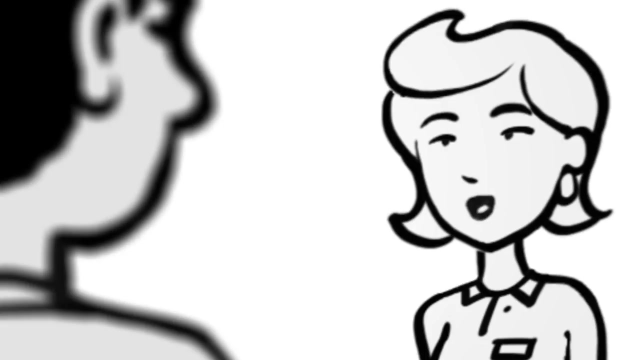 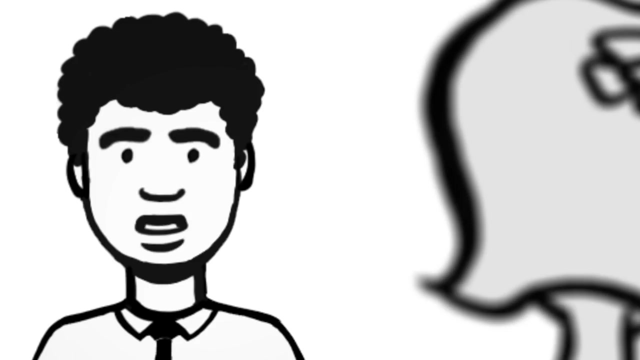 attacks, and so it's not just about defending the perimeter, but ultimately detecting attack and hoping to mitigate the consequences and the duration. can they get to the actual target? hello, I see that you selected continuous monitoring. are you also interested in response planning and analysis? not today. we already have an existing cyber. 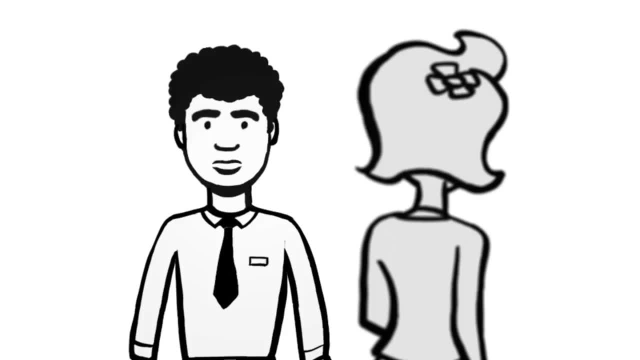 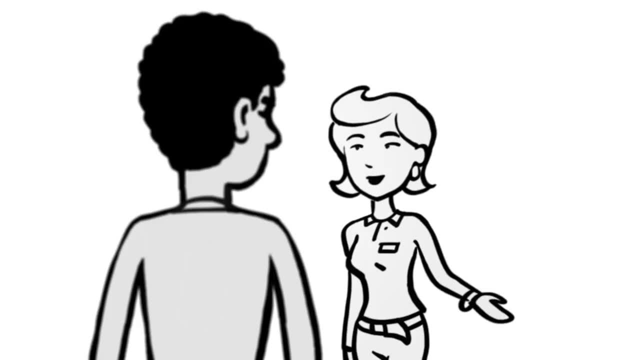 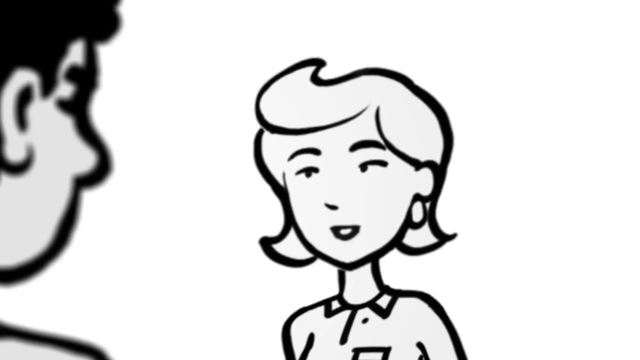 security risk practice, so we're only looking to add a few new categories at this time. excellent, the framework is designed with exactly that type of flexibility. it allows you to choose what works for your particular risk disposition and business. customize it to best suit your needs. have a nice day, sir.